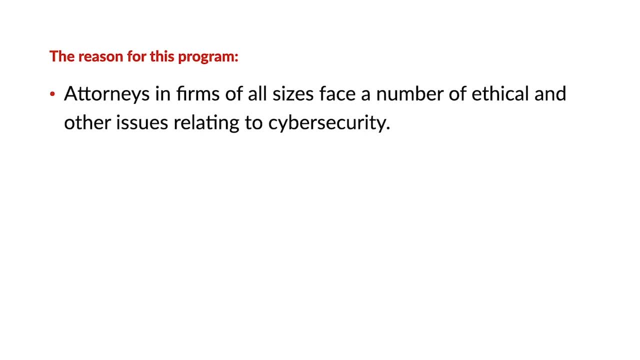 issues relating to cybersecurity, particularly in these days of data being breached and hackers running wild with the data that does get breached, It's very important for companies, law firms, lawyers, to preserve the confidentiality and the security of their clients' data Companies and even law firms themselves are often valuable. 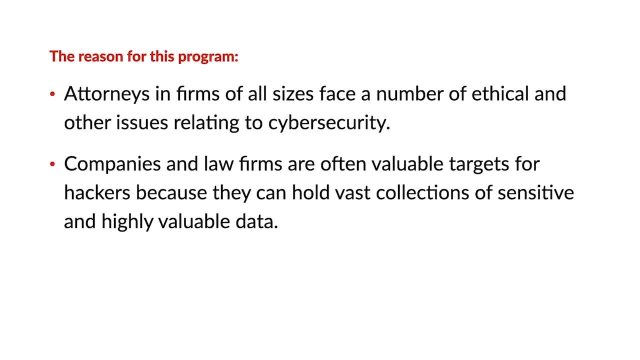 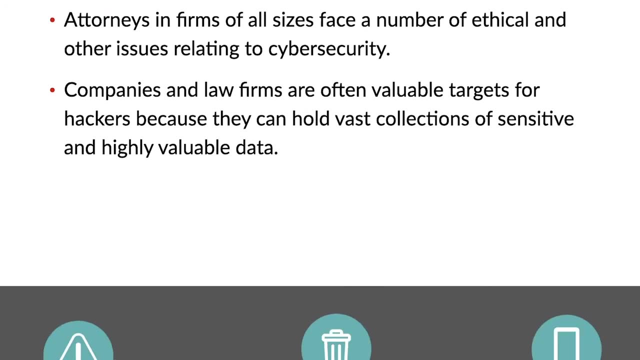 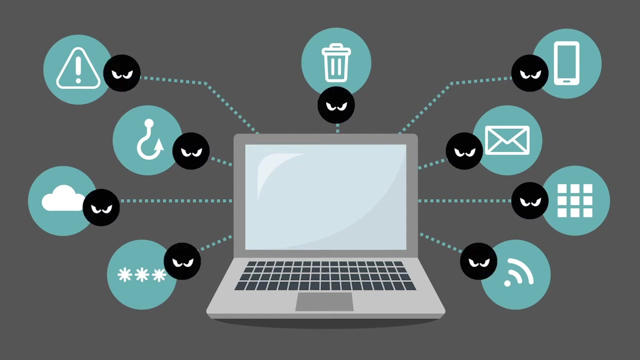 targets for hackers because they can hold vast collections of sensitive and highly valuable data, such as IP data, non-public information relating to public companies and other types of data. There are security threats that come from all different sorts of places, including individual hackers and international cybercriminals. the types of 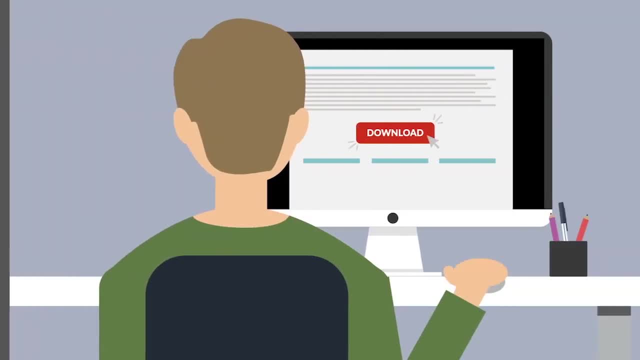 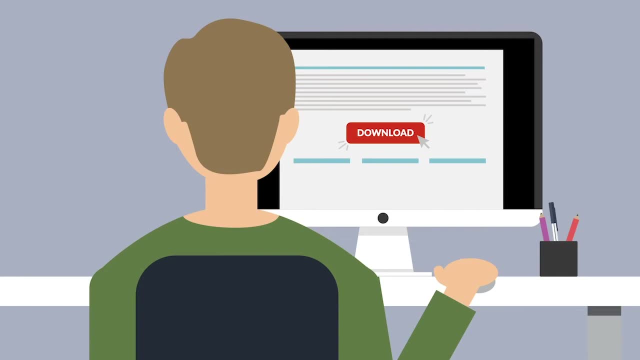 bad actors that get a lot of press. But it's not just the outside world that companies and lawyers need to be concerned about. There's also a company's own employees that could be allies at least, and they could internally breach data either maliciously or negligently. 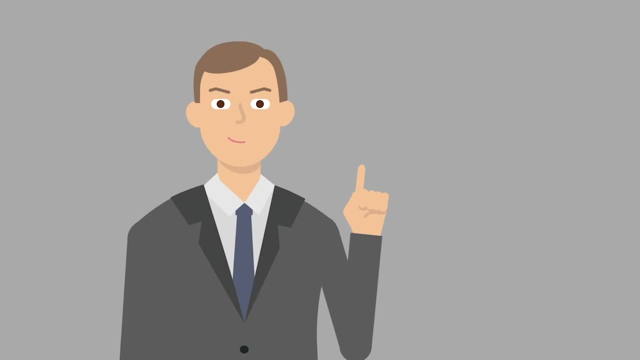 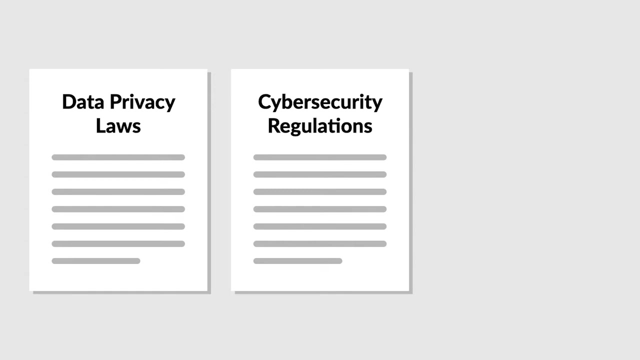 First, in connection with figuring out how lawyers should keep their clients and their companies and firms as secure as reasonably possible, it first helps to understand what types of data needs to remain secure. There are data privacy laws and cybersecurity regulations, regulations that protect certain types of data. In addition, your company or your firm 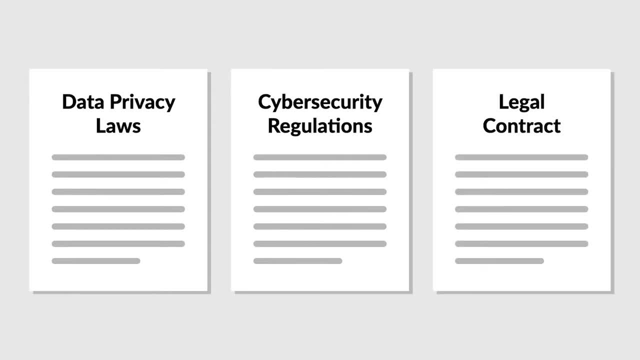 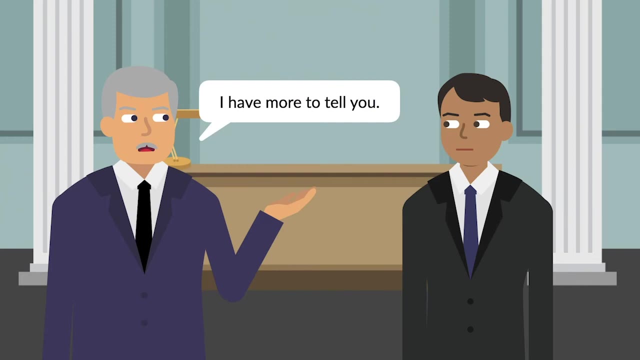 may have contractual obligations to keep other types of data secure, even if that type of information is not protected by laws or regulations. As a lawyer, you'll have clients who share all types of data with you, whether it be protected data under law or data that.